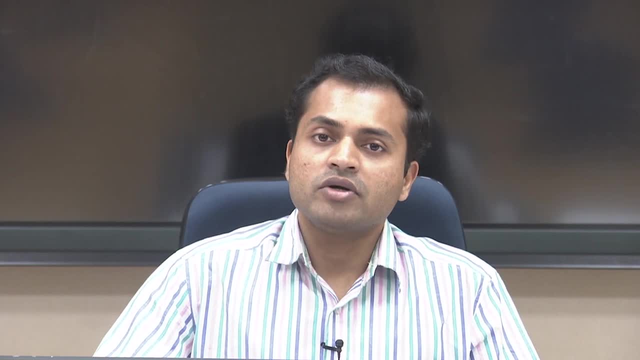 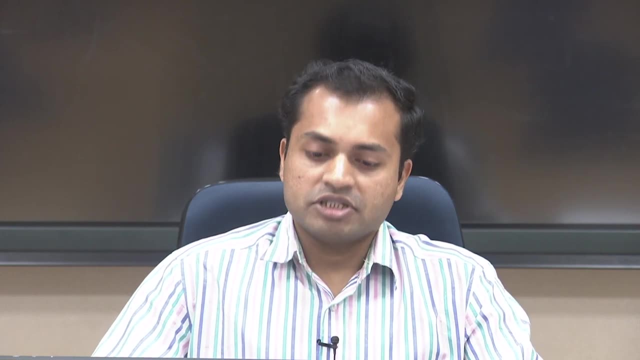 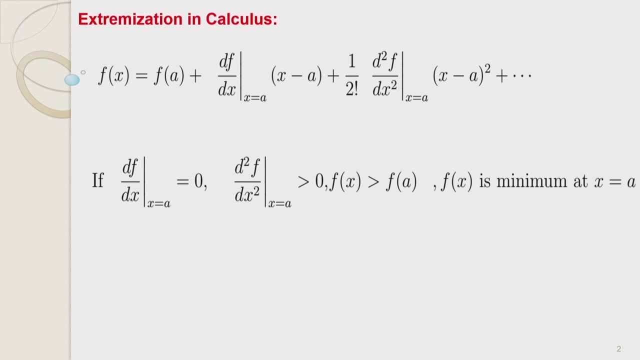 Let us look at the further theory of finite element method. Let us start with our ordinary calculus, where some function- f, x- can be expressed, as in Taylor series, in this form: Now suppose we draw a function which is minimum at a certain point, a Now we know from our ordinary 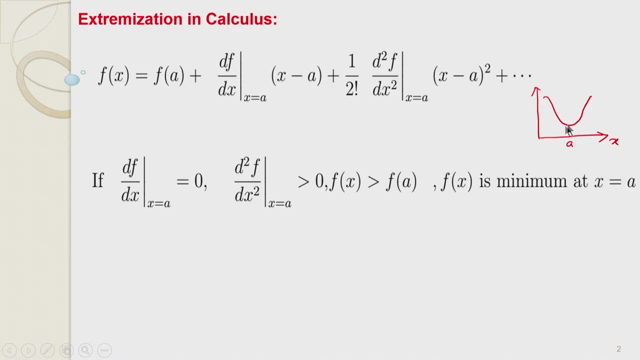 calculus that at this point, d, f, d x, the first order derivative is 0.. Therefore we will draw a function. f x can be expressed, as in Taylor series, in this form: and the derivative of f x is 0.. The derivative of f x is negative at f x. in the other form, This derivative of f x will: 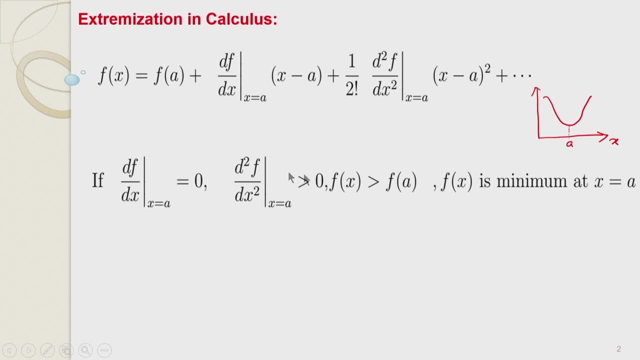 be zero and f x will be negative at f x. in the other form The derivative of f x can be expressed: and also the second order derivative has to be greater than equal to 0. So if you see in the Taylor series the higher order term, that approximately goes to 0 in the vicinity. 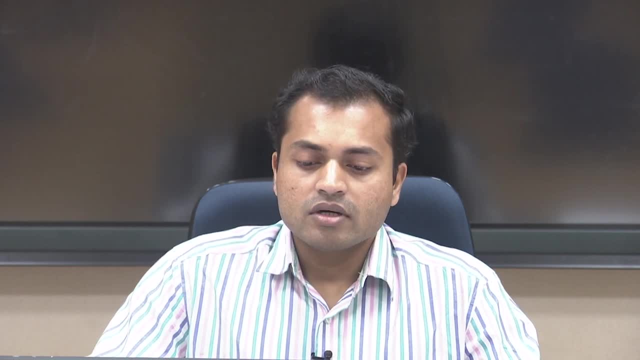 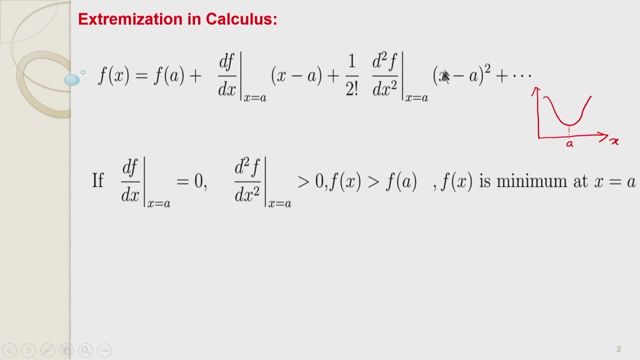 of point A. So the first term is 0 and because the second term is greater than 0, so f x is greater than f A. Hence, at x equal to A, the function is minimum. This is the relation between this explanation with Taylor series and the graphs. So this is our f x and this. 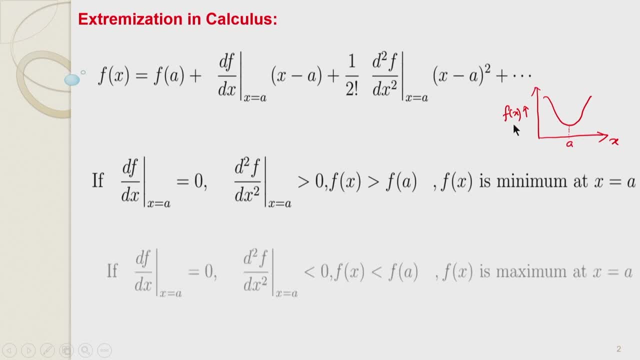 f x. Now, similarly, if the first order derivative is 0 and this is less than 0, then this quantity is 0. This second quantity is negative and all higher order term we can neglect in the close vicinity of x equal to A. Hence the function f A is less than or equal to f x. 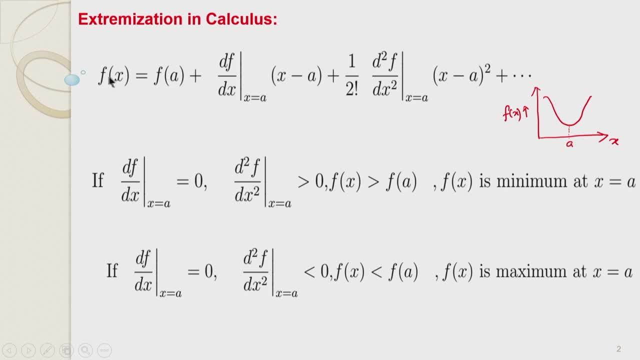 that is at point A is greater than f x for the point close to A. Hence f x is maximum at x equal to A. So this first derivative, equal to 0, is the necessary condition to be extremum, and the second derivative, if it is greater than 0, then that is the sufficient. 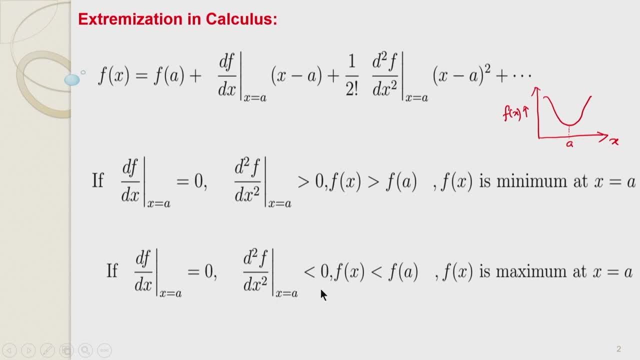 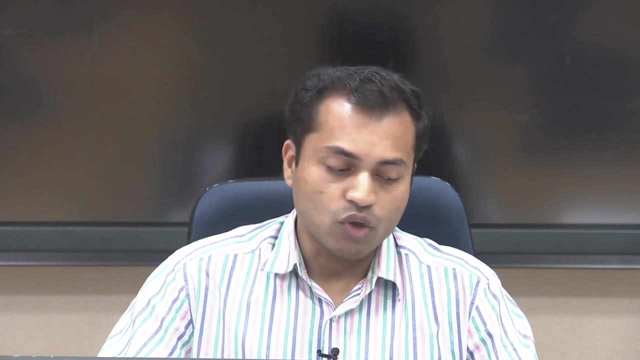 condition For f x to be minimum, and if it is less than 0, then that is the sufficient condition for f? x to be maximum at x equal to A. This is all about our ordinary calculus, which we already know. Now, in variational calculus we come across a new quantity which is called functional. 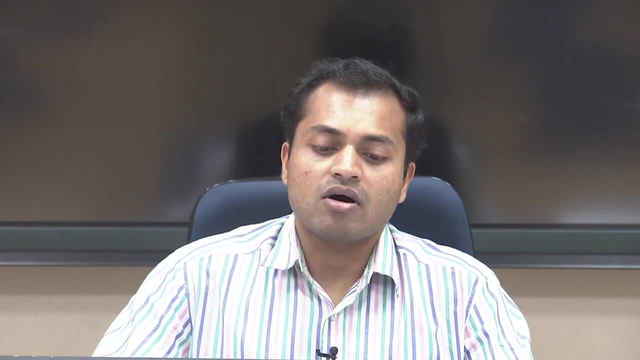 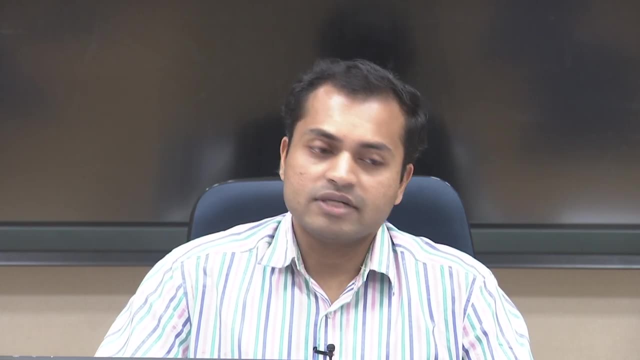 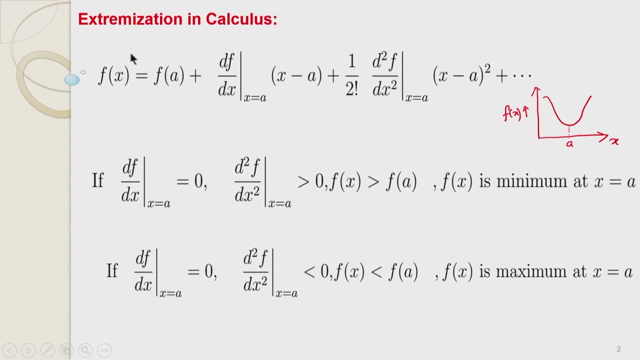 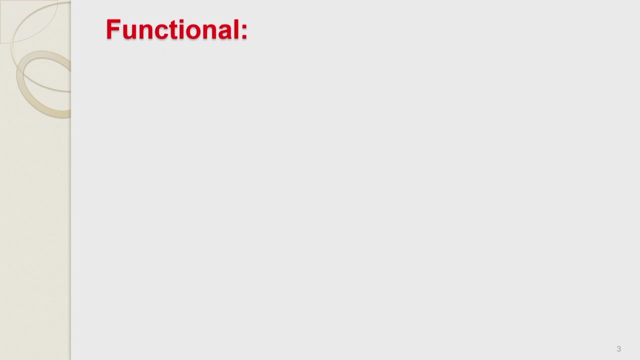 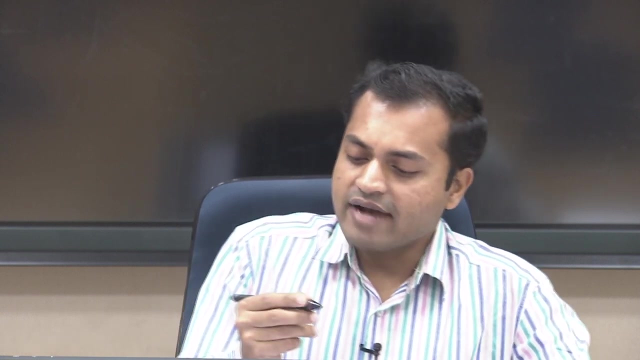 Now what is functional? In ordinary calculus the function is only dependent on the independent variable x. Some time in physics it can happen that some function is dependent on another function. We can write some very simple form, for example, that is: i x 1 to. 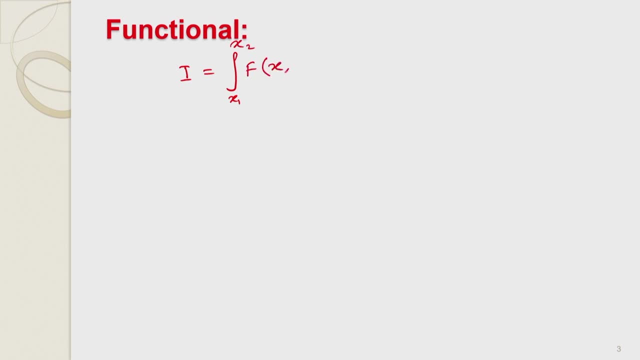 x, 2.. Now this is a quantity which is dependent on independent variable x and also a dependent variable y and its derivative 1.. So this is the independent variable x and also a dependent variable y, So we can write some very simple form for this. For example, this is the function. 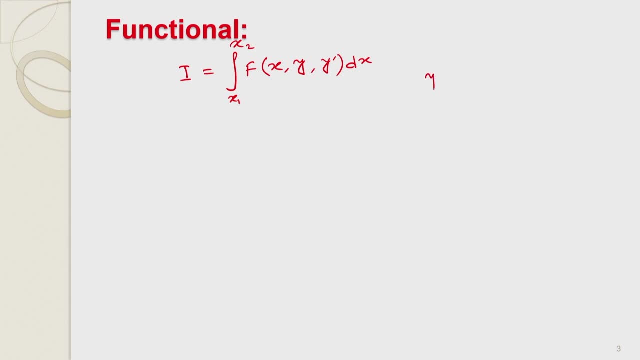 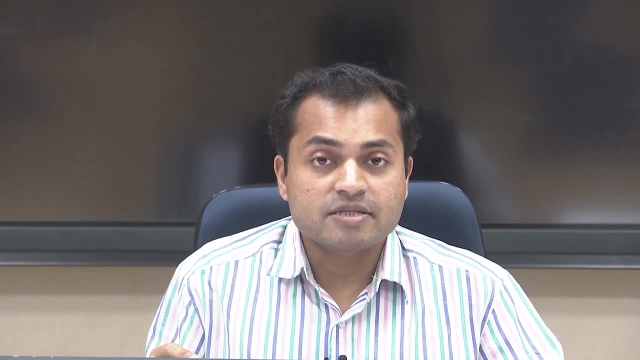 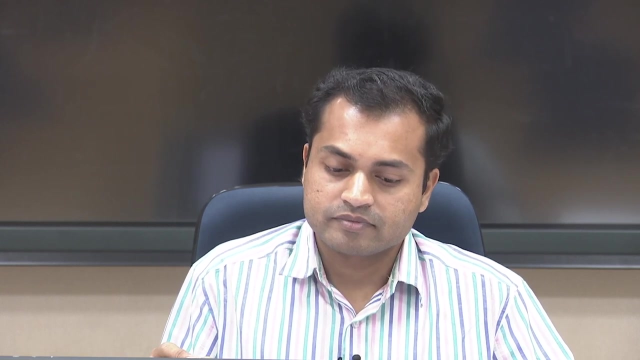 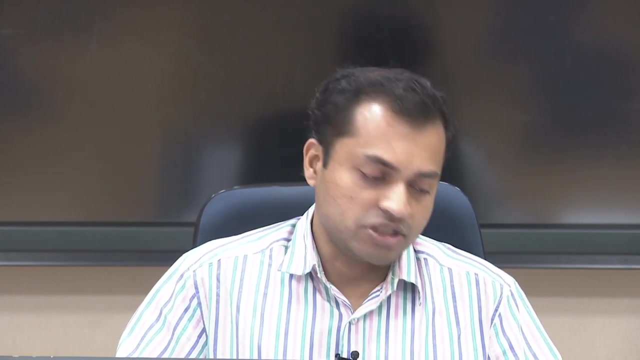 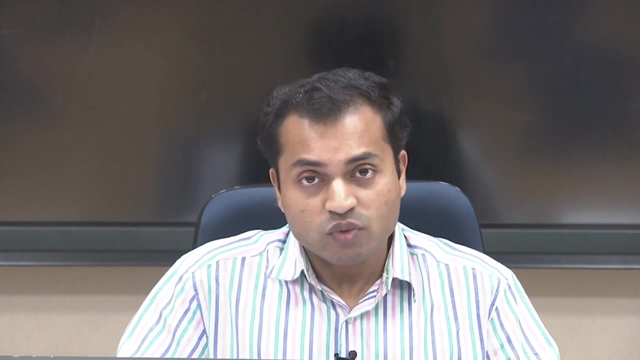 and its derivative y prime, where y is also function of x. Such quantity, which is dependent on independent variable as well as on dependent variables, are called functional. In Nutshell we can say: a functional is nothing but a function of functions. Let me explain this concept of functional with one example, that is, Brachystroken problem. 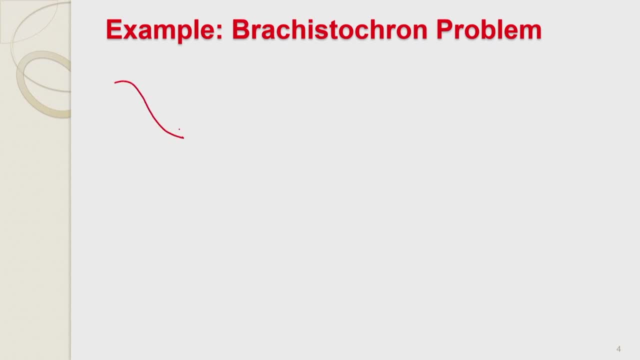 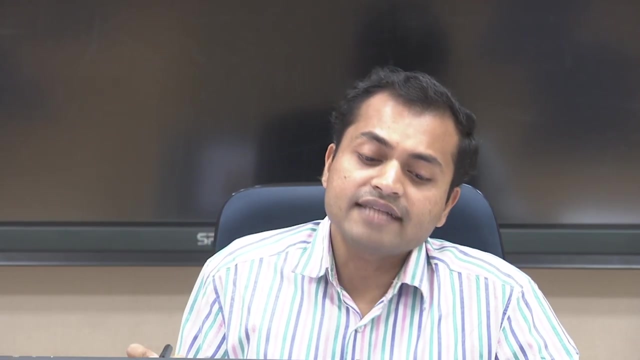 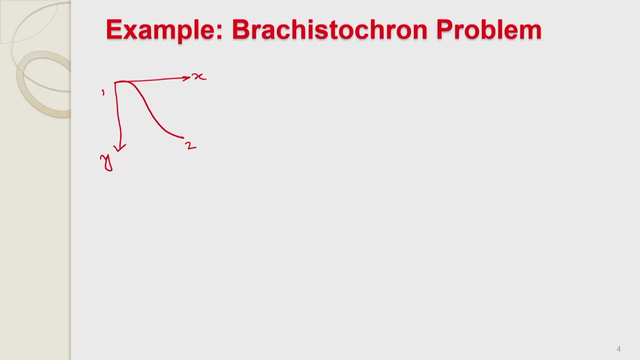 Suppose we want to go from point 1 to point 2 with any path under the action of gravity and we set our origin at point 1.. Now, under the action of gravity, if the point pass about a depth y, then its velocity v is. 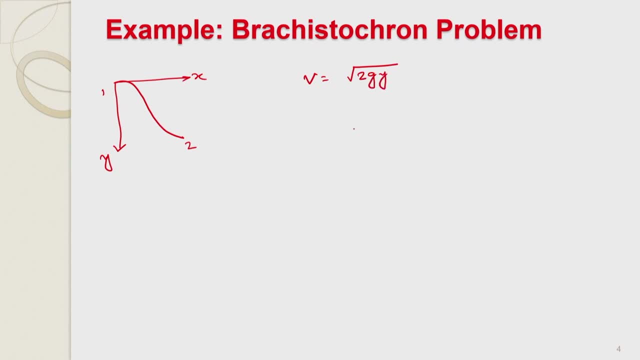 root over 2, g, y. Now, when the particle travel a certain distance- differential distance d s- then the time is d s by v. Now the total time to travel from point 1 to point 2 can be obtained by integrating from x 1 to x 2.. This is our total time Now. 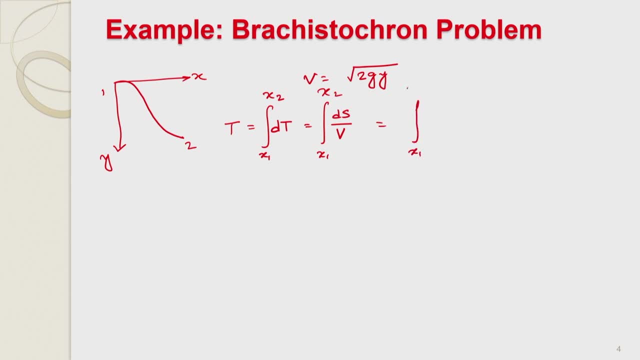 d s can be written as: And our v is root over 2 g y. Now we can write this as N: showcase v as root over 2 g y. In methods error there is some error inhua function told. Let me physically right this. 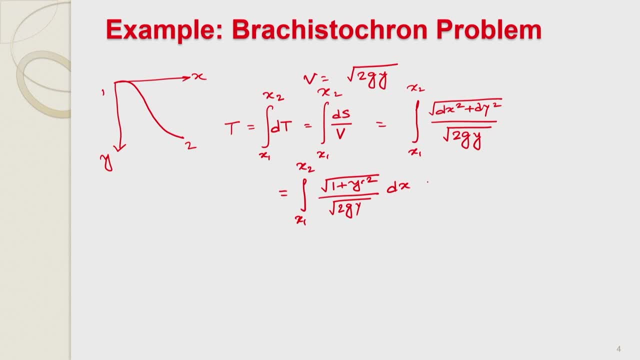 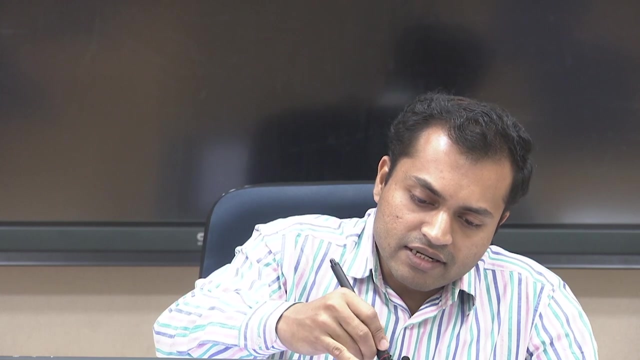 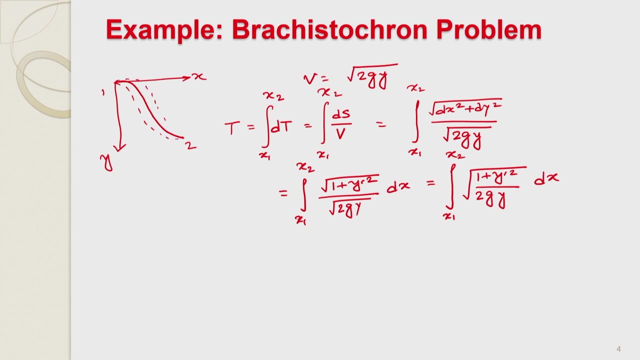 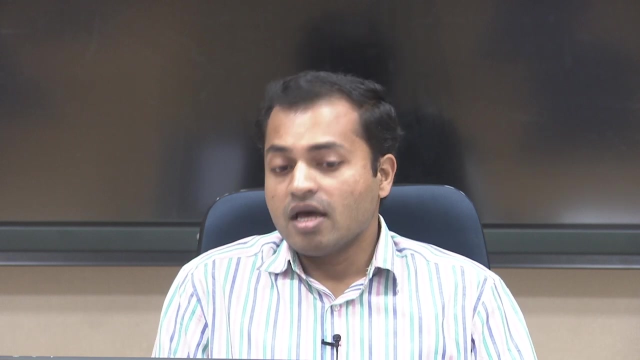 you here v. Our v is Now: we want to find the path. there are several path possible between point 1 and point 2.. It can be straight line also. now, the straight line between point 1 and point 2 is the path which has minimum distance. 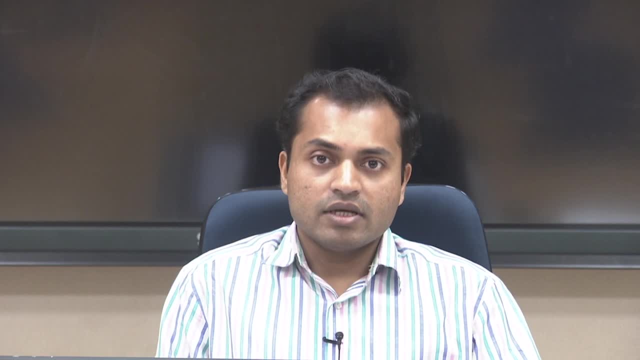 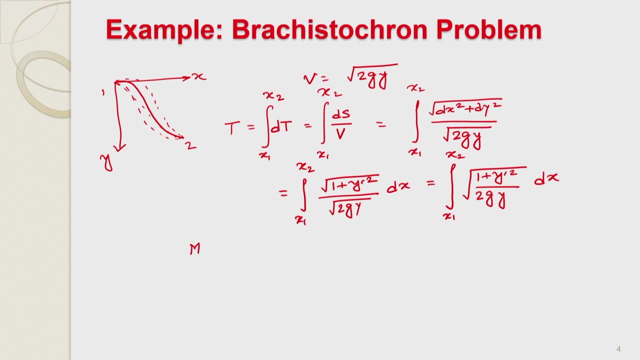 We want to find a path for which it takes the minimum time. so we want to find y, x such that, If it minimize over y, this functional t. so here you can see, this functional is dependent on y As well as y prime, where both are function of x. 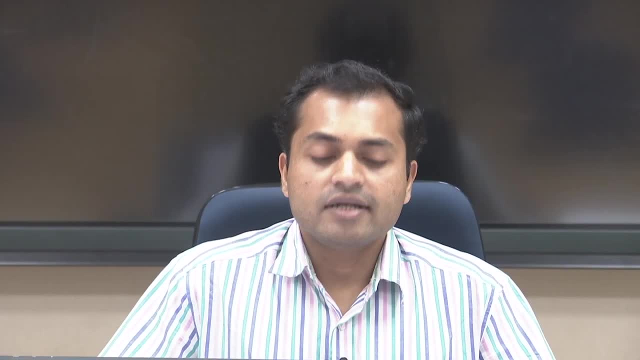 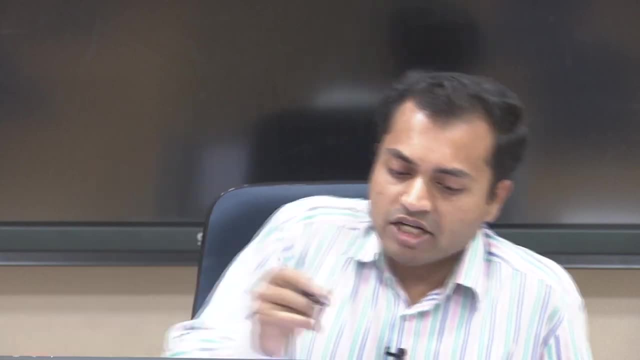 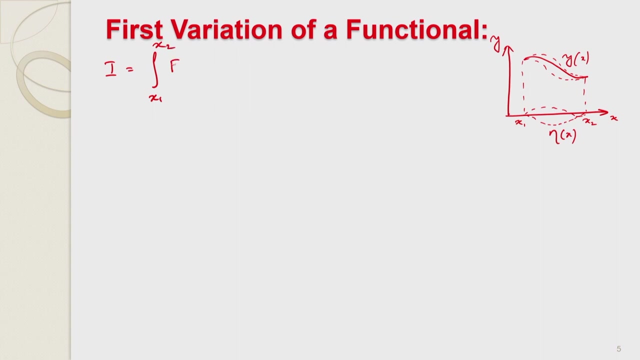 In the next section we will learn about first variation of a functional. So one functional can be written as: 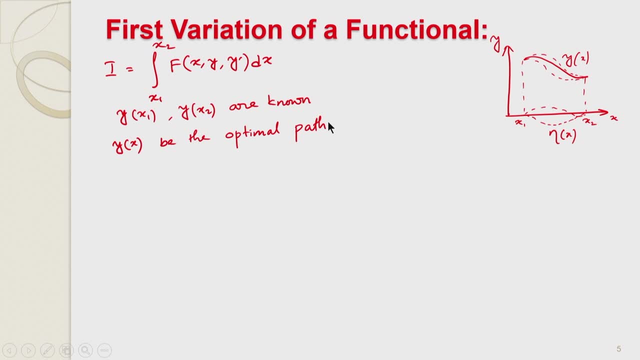 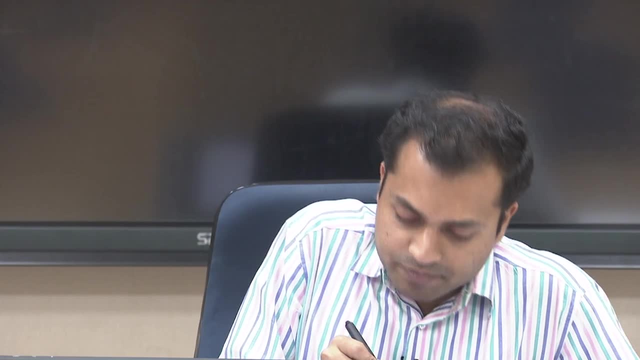 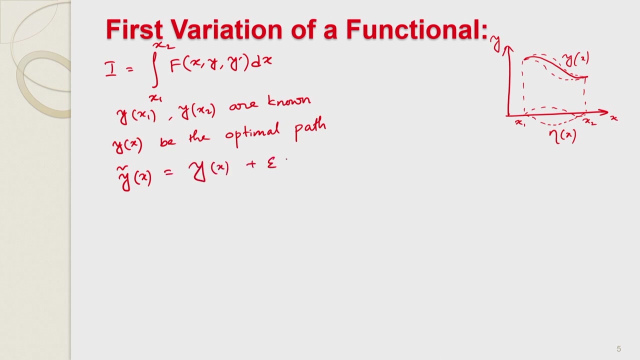 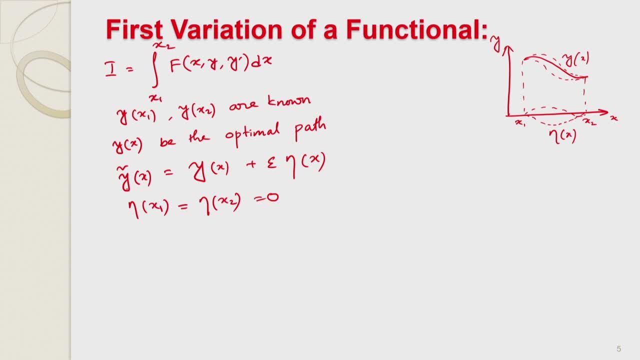 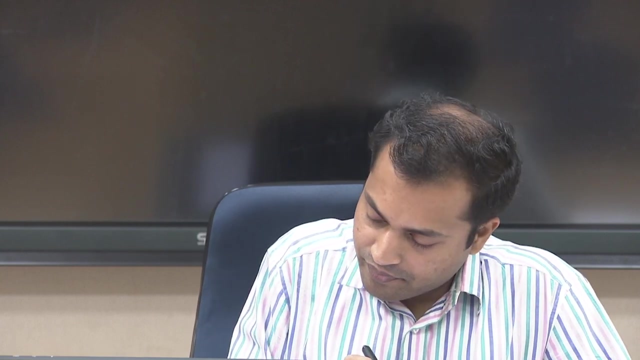 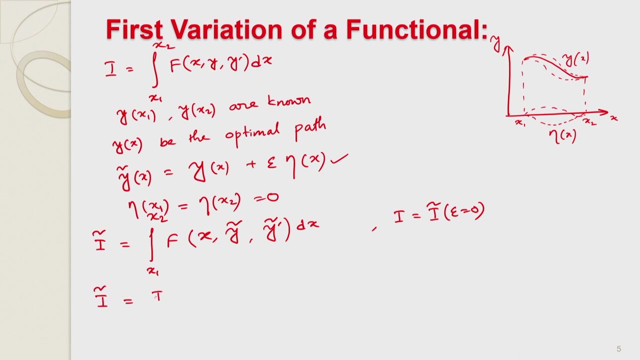 So i tilde to be extreme at epsilon equal to 0, that is i. to be extreme at epsilon equal to extremum, The necessary condition is the first variation, that is, should be 0.. So this: 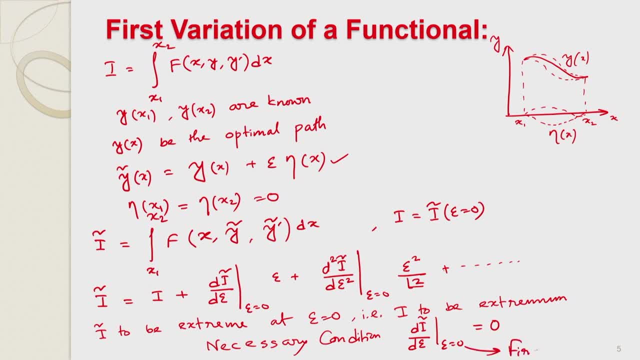 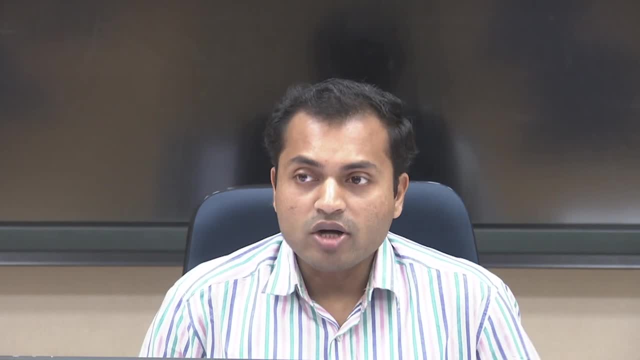 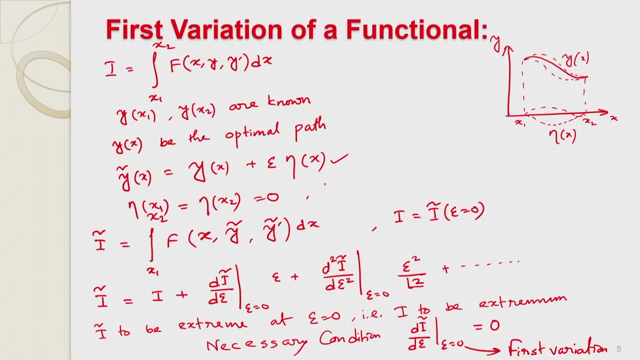 is called first variation of a functional. Now, one important thing to note is that choice of eta x is arbitrary. The only thing that eta x should satisfy, that is this two. at this two point, it should be 0, because y is specified. 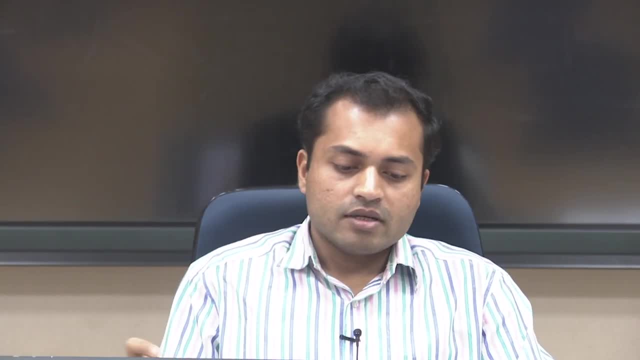 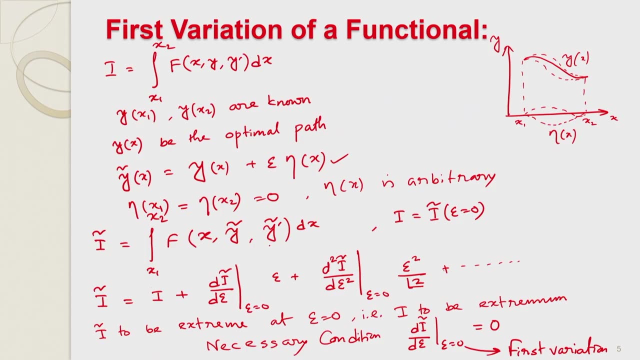 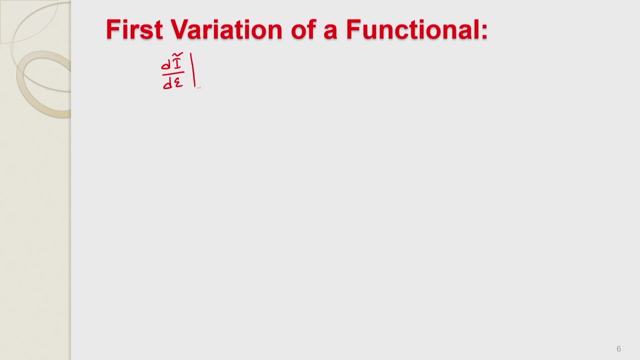 at this two point. Now, if you see that i tilde is dependent on x, y tilde and y tilde prime. Hence this first variation can be written using chain rule in following form: Because it is dependent on: 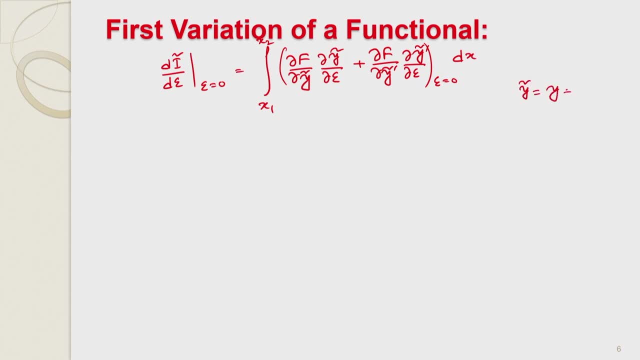 gold . . . . . � But if you notice that X z equal to 0 plus apostles theta can be written. This is what that we want to do. . . . . . . . . . . Now, at epsilon equal to 0 y tilde is nothing but y. 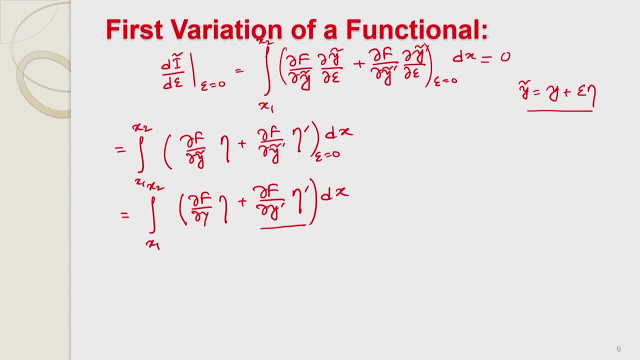 Now the necessary condition is this: first variation has to be equal to 0. And we have arbitrary eta x, that is, we can choose any eta x. It should satisfy that at x1 and x2 it should be 0, because y is specified at x1 and x2.. 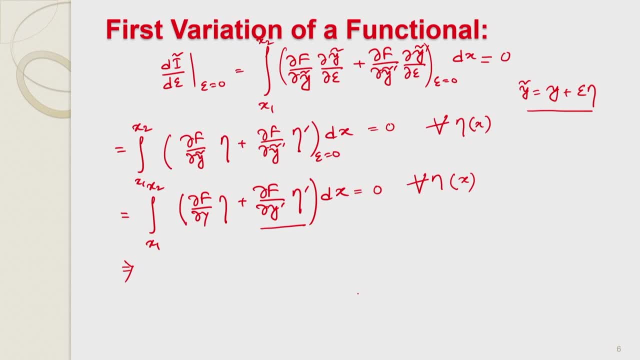 So this term we can do integration by parts. 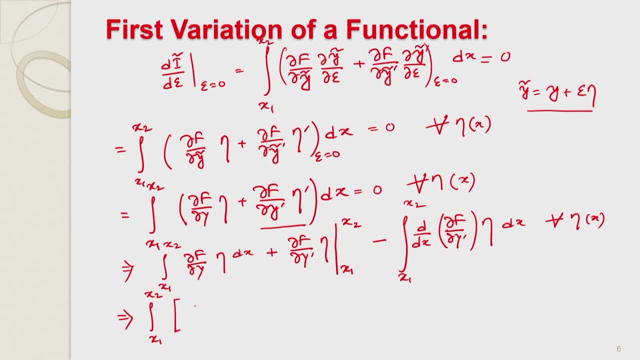 Now on boundary, because eta is 0 at x 1 and x 2, as our function y is prescribed there, so this will be 0, the boundary term will be 0, so this equal to 0.. 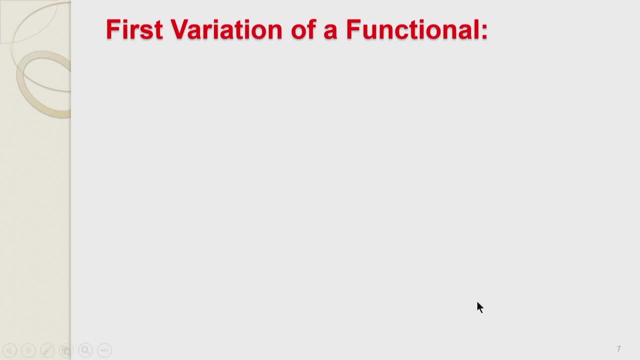 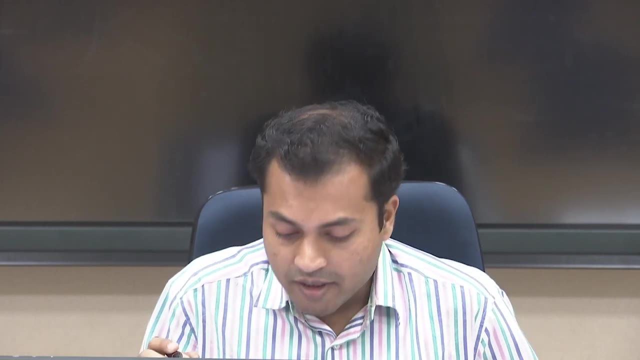 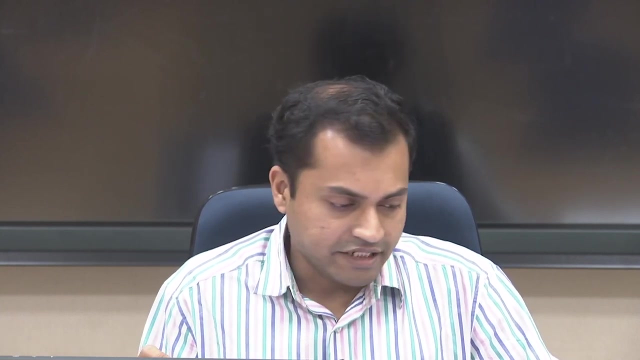 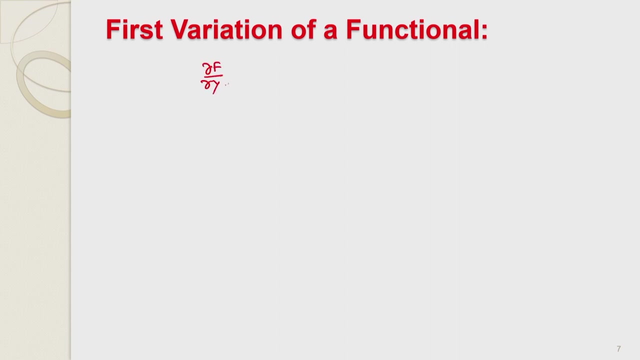 This is for any arbitrary eta x. Now, using this arbitrariness, because it is true for any eta x, We can wrestle that a set of problems. the problem when this class breaks down into parts, write. this equation is called Euler Lagrange equation. 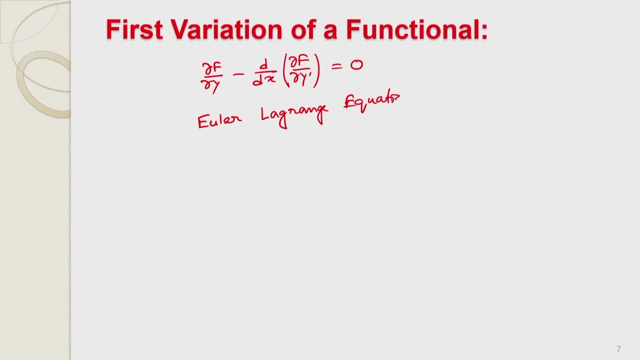 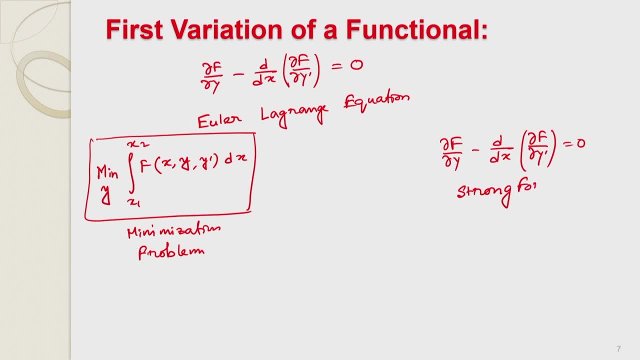 This is also called the strong form. Now, this differential equation is valid for all point x between x 1 and x 2.. Now, regarding boundary conditions, we have started with that y is prescribed at x 1 and x 2.. 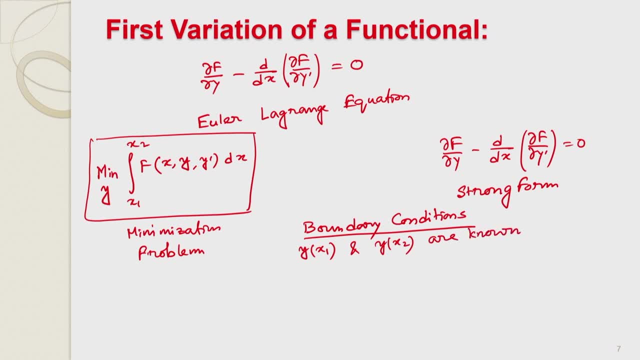 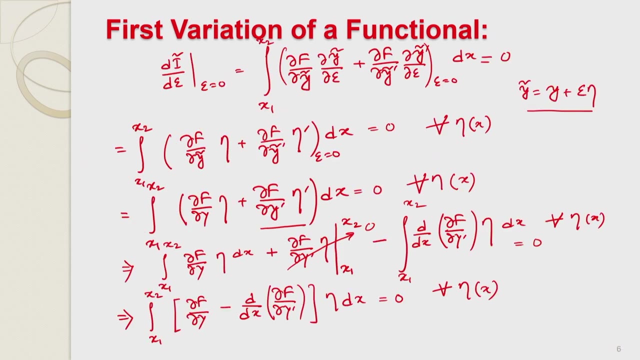 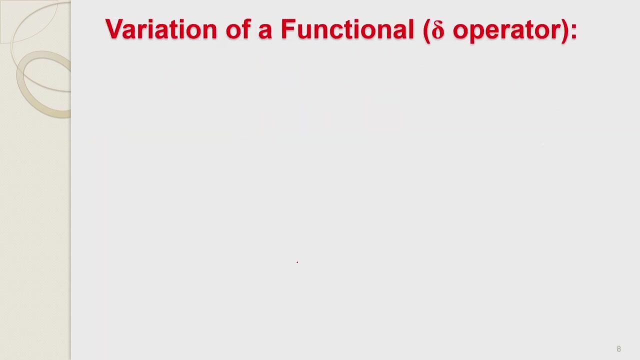 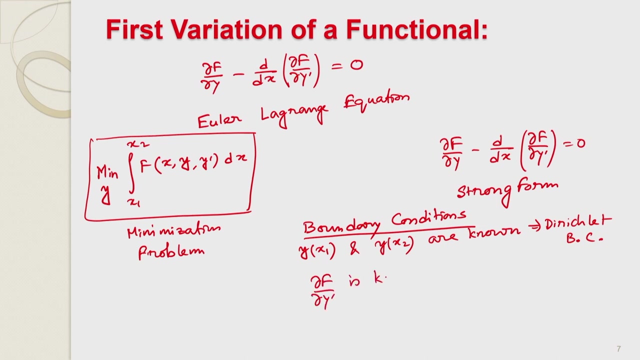 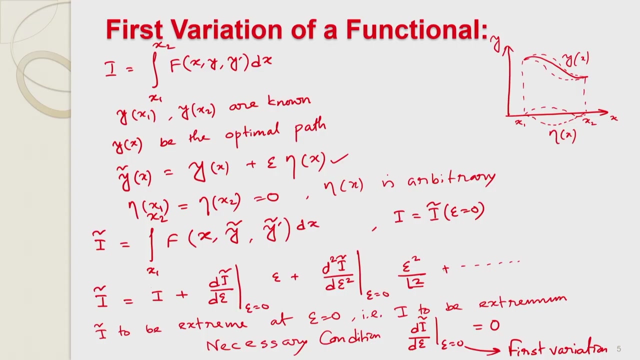 Thus, to summarize: for a given functional, we can expand in Taylor series: The first order derivative of the functional is called first variation of that functional. Now for i tilde to be extremum, this first variation should be 0.. 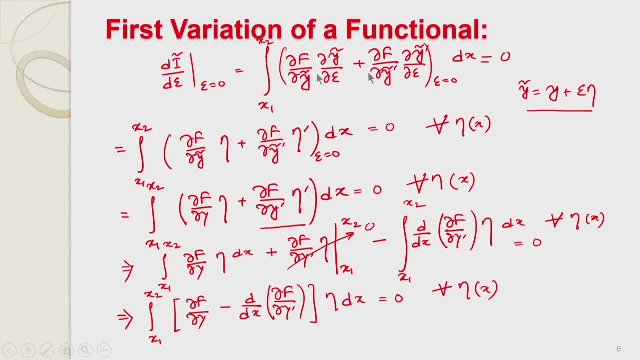 And because the functional is dependent on y and y prime. hence this first variation can be expanded using chain rule And where y tilde is y plus epsilon eta. therefore we can write this as eta and this as eta prime. 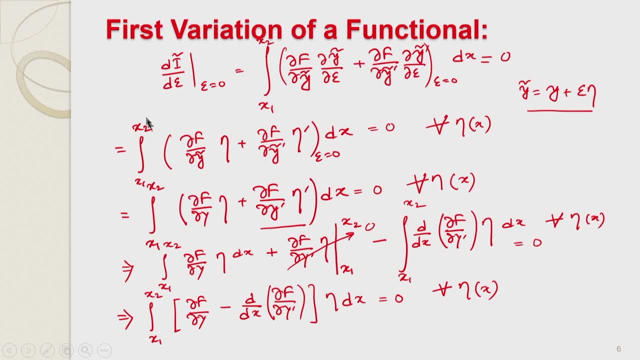 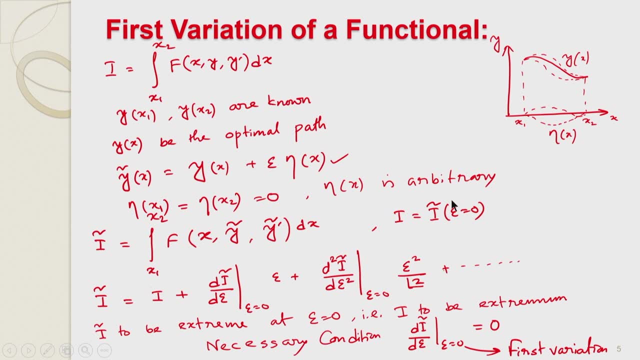 And this entire derivation is for any arbitrary eta. There is no particular choice of eta. The only condition eta should satisfy that at x 1 and x 2, it should be 0. Now, therefore, this is true for all eta x. 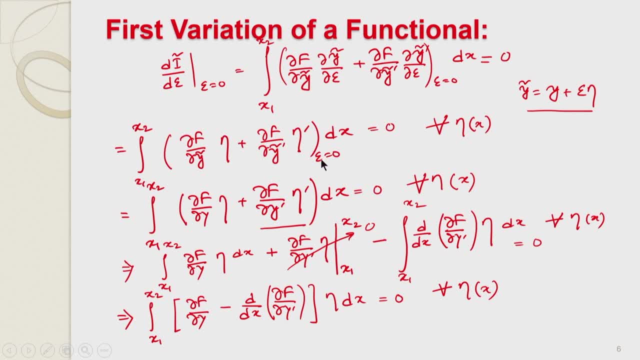 Now, because at epsilon equal to 0, it become 1.. Because at epsilon equal to 0, it become y and y prime. After that we do integration by parts of this second term, and because eta is 0 at x. 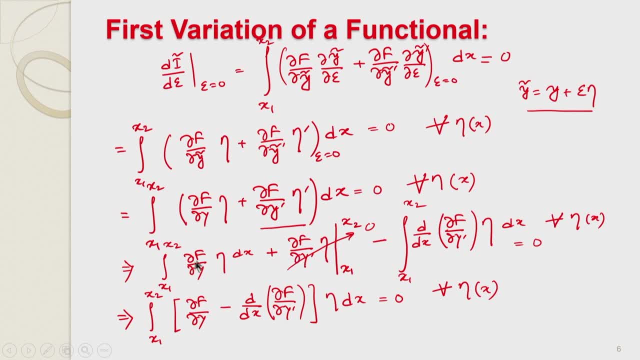 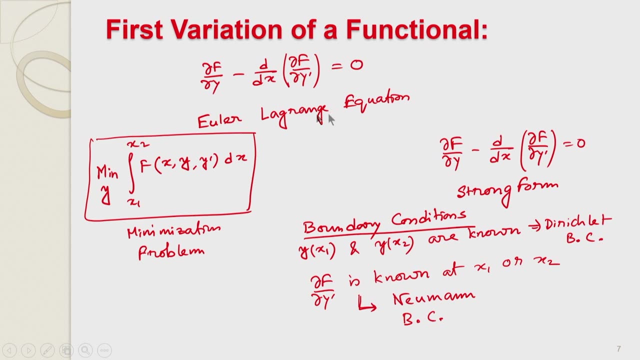 1 and x 2, this term goes to 0.. And finally, we have this expression for any arbitrary eta And because of arbitrary eta, we can write this as equal to 0, which is the Euler Lagrange equation. 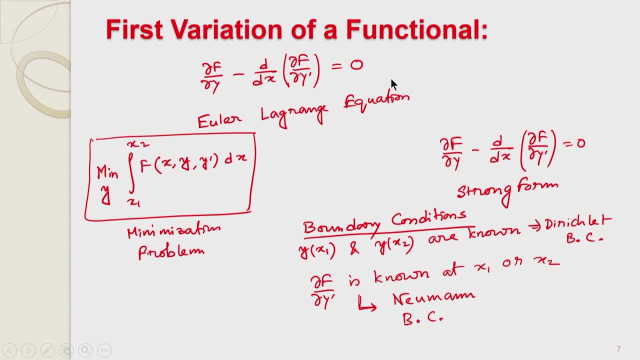 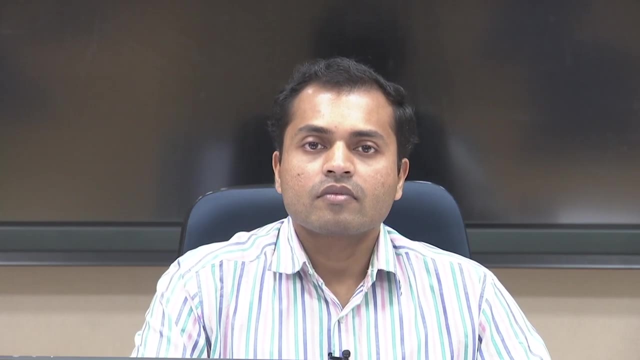 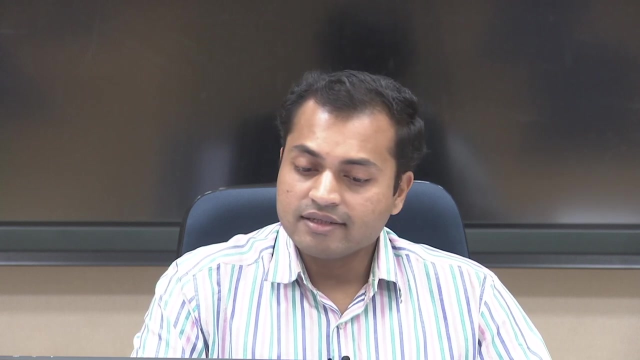 And this is the differential equation which describe the same problem as minimizing this functional. And also there are two type of boundary condition: Dirichlet and Neumann. We will see variation of a functional that can be expressed using delta operator. 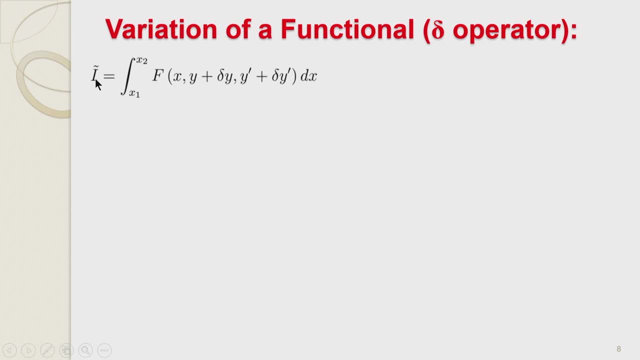 So the functional i tilde, that is the varied functional, we can write as y plus delta y. This delta y is nothing but variation of y. Now this is the variation of the functional. that should be equal to 0 for i tilde to be. 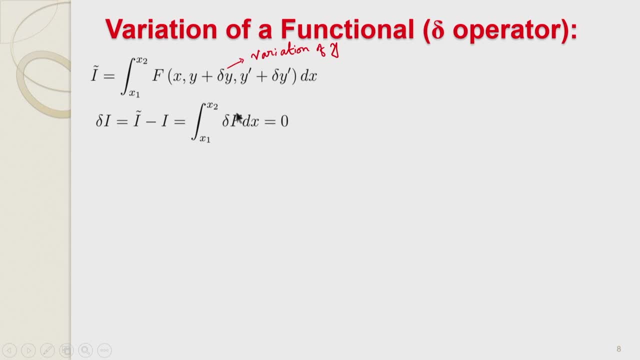 extremum. Now this delta f can be written as this expression: This is the chain rule, because f is dependent on y and y prime. Now delta y is variation of y and it is variation of y prime. Then this second term can be written using integration by parts. 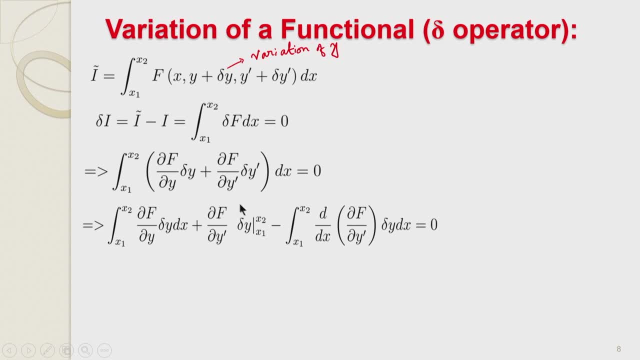 So this is the boundary term. Now we can combine the domain term and the boundary term. Now, if y is prescribed at x 1 or x 2, then delta y is 0. that is the Dirichlet boundary. 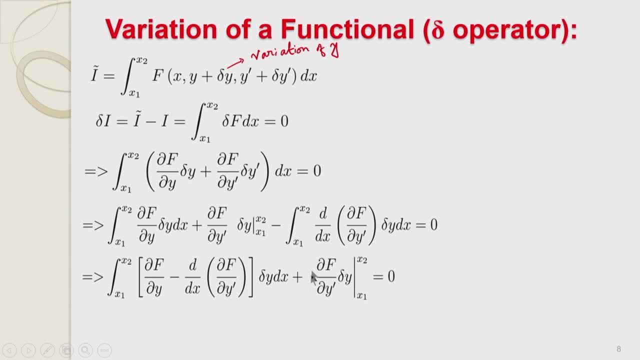 condition. The other boundary condition can be del f, del y, prime. that is Neumann boundary condition. All these are for any arbitrary variation, that is arbitrary delta y. So this arbitrariness, we can write this equation to be 0.. 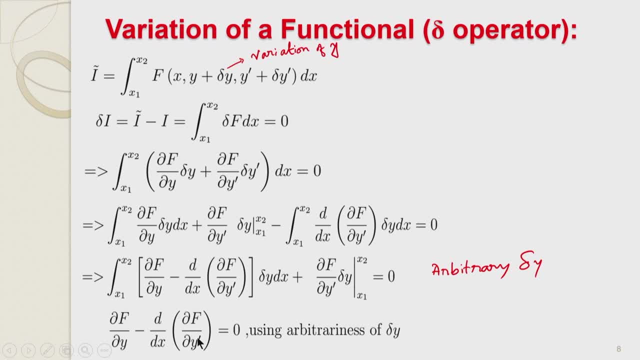 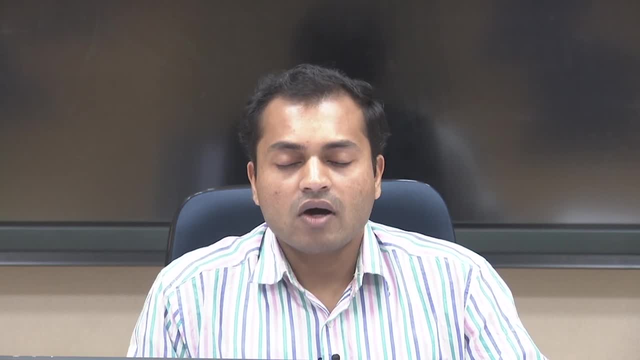 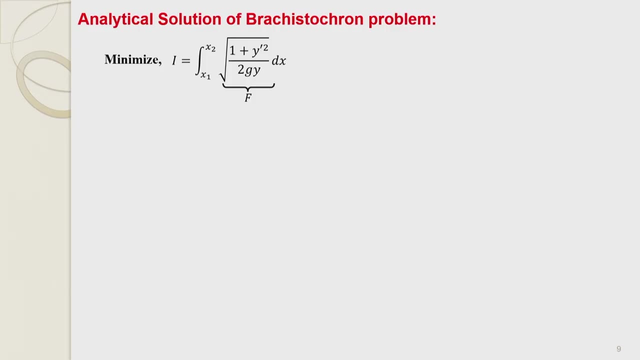 So we can derive this Euler Lagrange equation. Now we will apply this concept of first variation and Euler Lagrange equation to our previous problem, that is, Braki-Stroken problem. where we are, we have to minimize this functional. So you can see this is function of y and y prime. 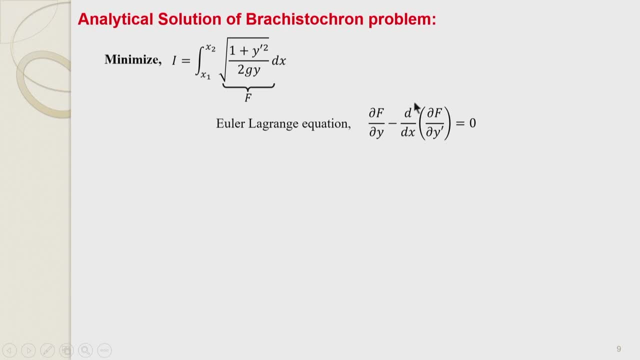 Now this is our Euler Lagrange equation, which we have derived taking first variation of this functional to be 0. Now if you substitute with this function f In this equation, you will get this expression and, with further simplification, the differential. 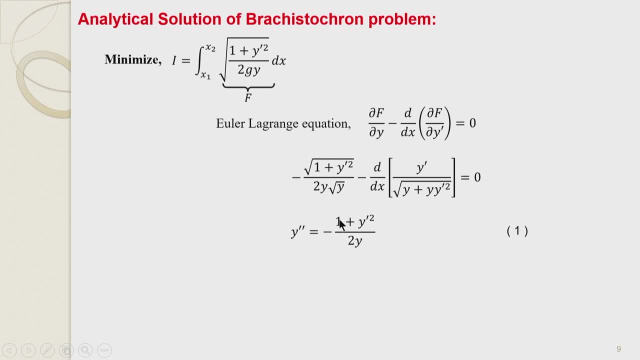 equation become: y double prime minus 1 plus y prime square by 2 y. So this is the differential equation which y has to satisfy at every point. x. Now just an extension. we are showing how to solve this differential equation. 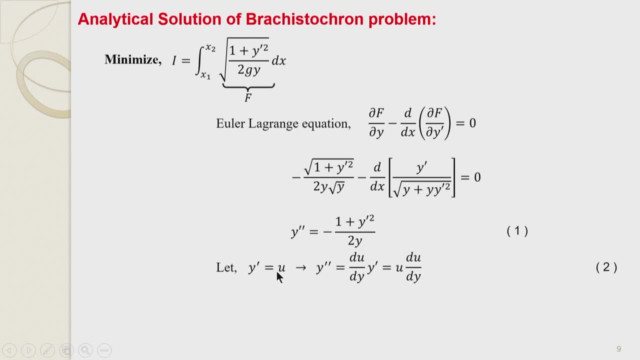 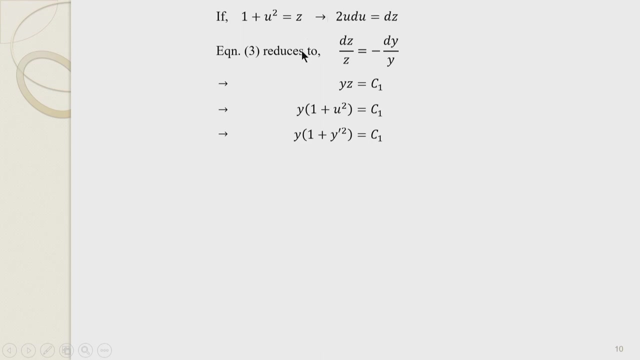 We can do this substitution: y prime equal to u. then we have this simplified y double prime is this: Now, if you replace this here, We have this expression: now, if you do further substitution, then equation 3 is this: and if you solve it, then y z is equal to c 1.. 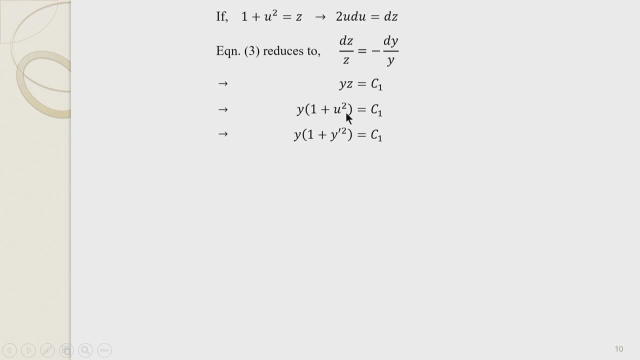 We replace z by 1 plus u square and u by y prime. Hence we can write this as y prime equal to this expression, that is, d, y, d, x. with further integration, we get this Now. here we can substitute using parametric expression as y equal to c, 1 sin square t. 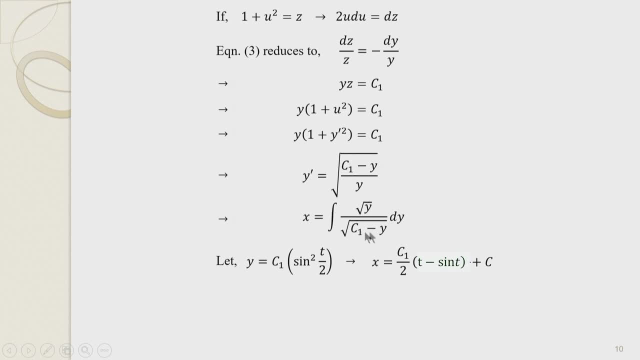 by 2.. If you do this substitution and if you can write also d y as a expression of d t, after that, if you do the integration, you have this form of x. Now this constant can be found. as you remember, we have chosen our origin at starting point. 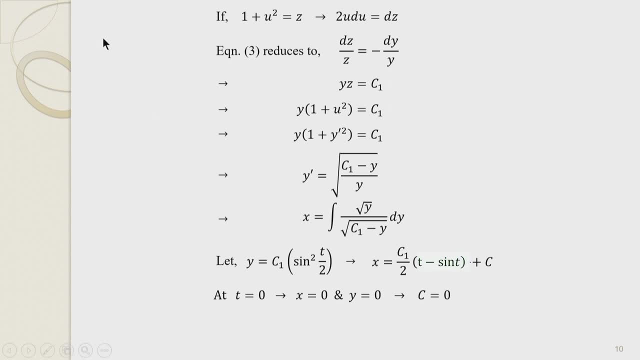 that is when x equal to 0, y equal to 0, and that is at starting. that is t equal to 0.. So from that condition we can find that c equal to 0. So then we have y equal to this and x equal to c, 1 by 2, 1 minus sin t. 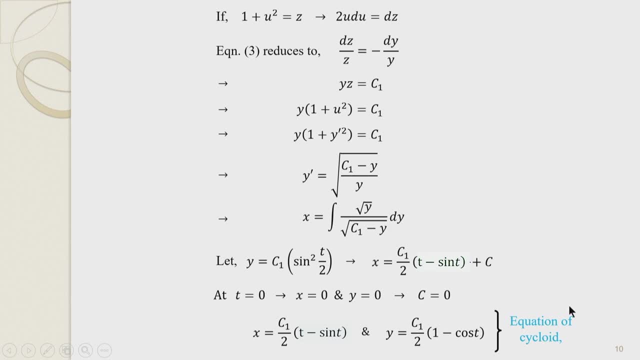 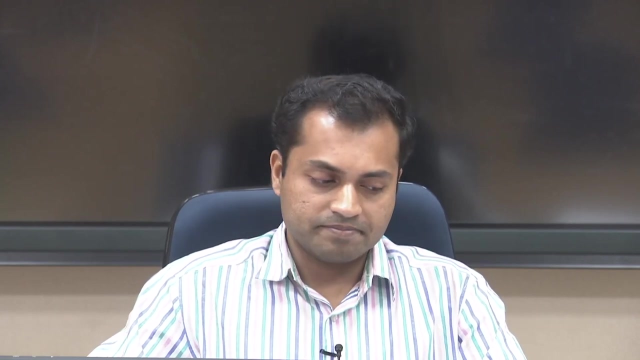 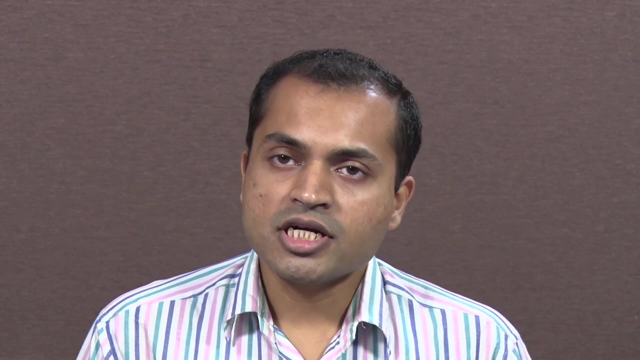 So this is the equation of cycloid. Hence this is the path which the particle if traverse, it takes the minimum time. So this is the solution of Bracke-Stroken problem. Now we will see how to minimize a functional which is functional. 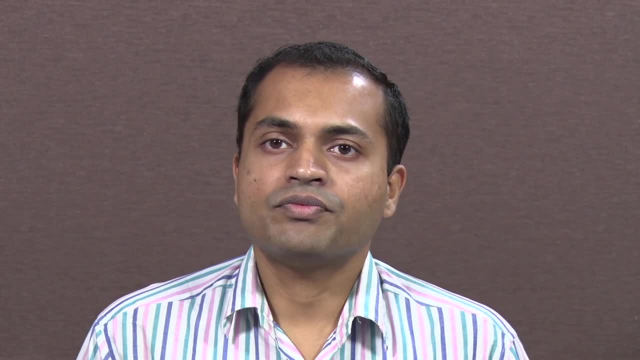 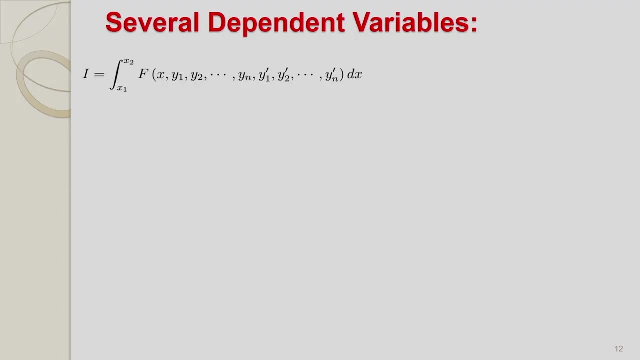 Which is function of several dependent variables. here if you see that functional i is dependent on n dependent variable y 1 to y n and their first order derivative, So y 1 to y n, all are function of independent variable x. we want to minimize this functional. 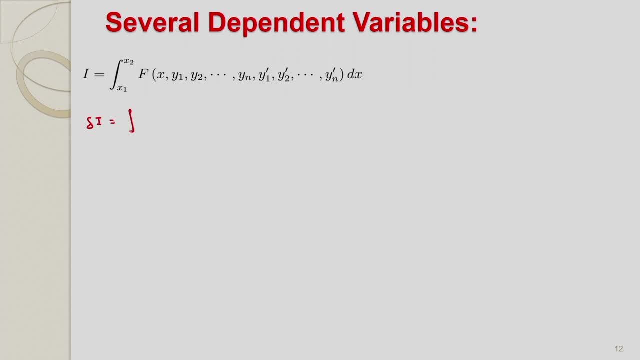 So the terms of several dependent variable. The similar way up to Yn. also, we have to consider the variation of their first order derivative. Thank you. 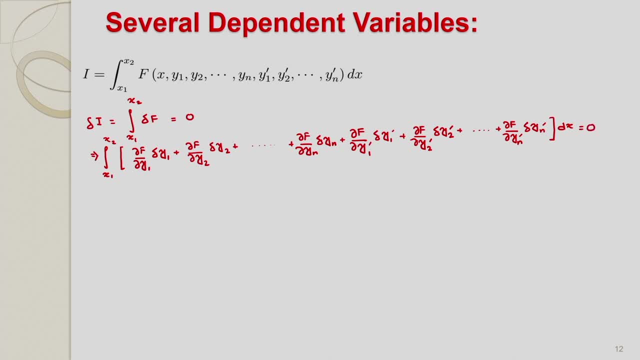 Now, using arbitrariness of variation, we can choose delta y2 to delta yn equal to 0 and and we use arbitrariness of delta y1.. Then we can write this as: 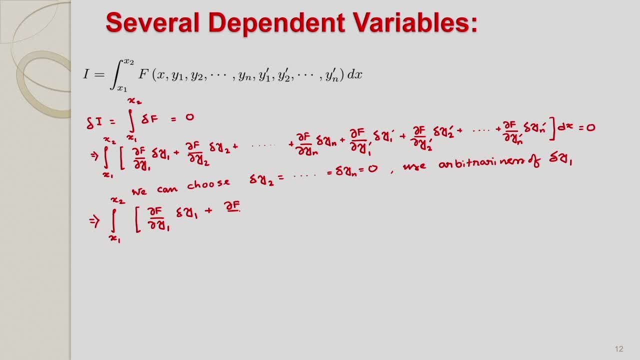 Now we can do integration by parts for this second term, and this is a constant integration. now we can see that integration by parts for this second term appears as seen in the 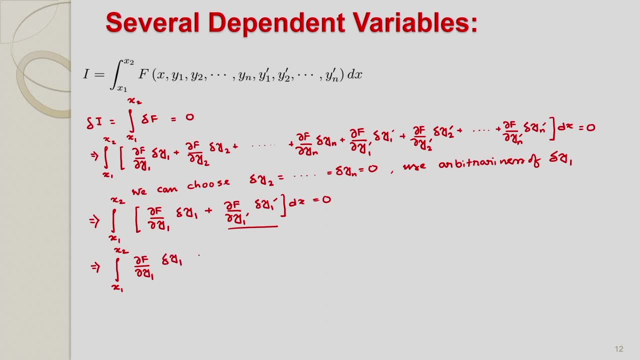 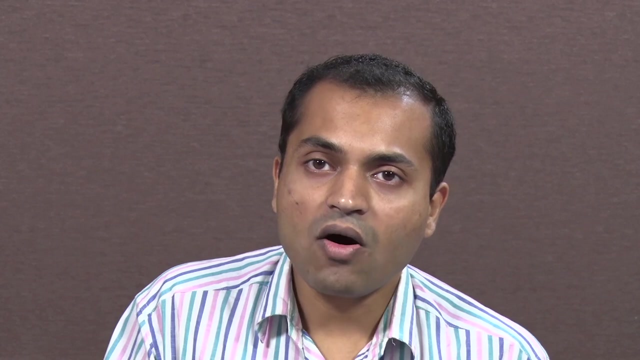 Thank you. Now we can combine domain terms with domain terms, So this boundary term will be decided based on essential and natural boundary condition on y1.. So we can use arbitrariness of delta y1.. Now this expression is true for all choice of delta y1.. 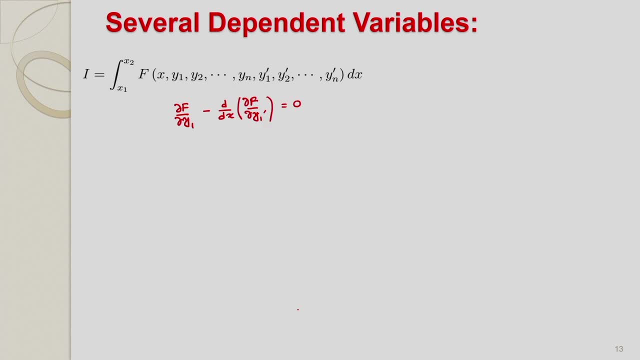 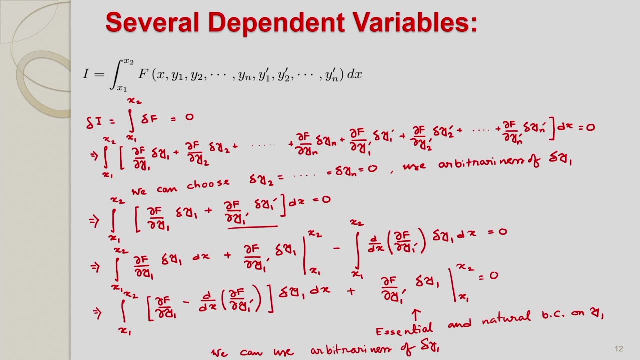 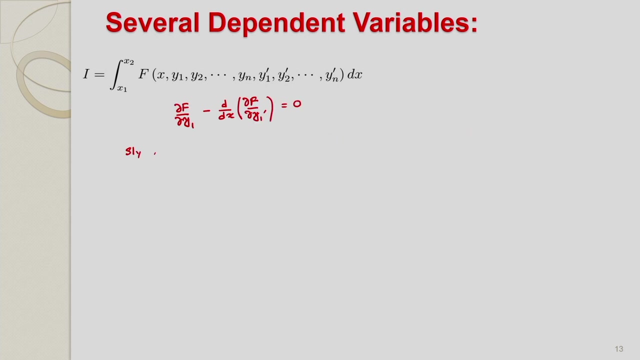 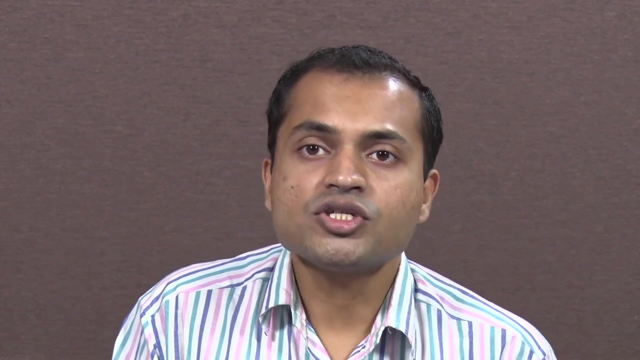 And we can write this equation Now. similarly, we can make other variation 0 other than delta y2 and in the similar way, we can write this differential equation with respect to delta o equation with respect to y2.. In this way, for various choice of delta y1 to delta yn. 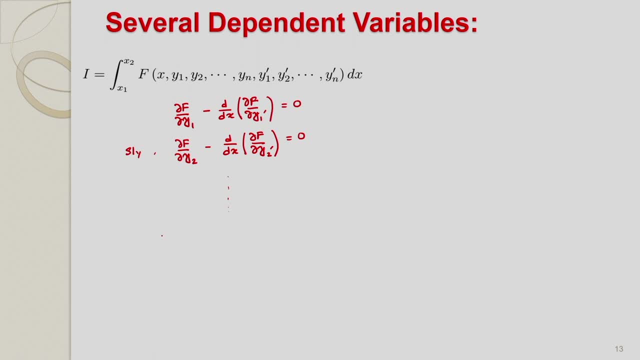 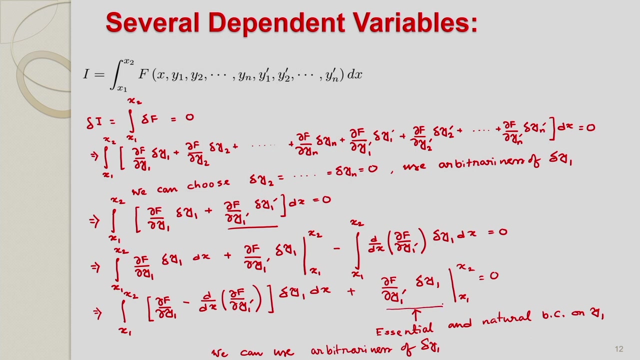 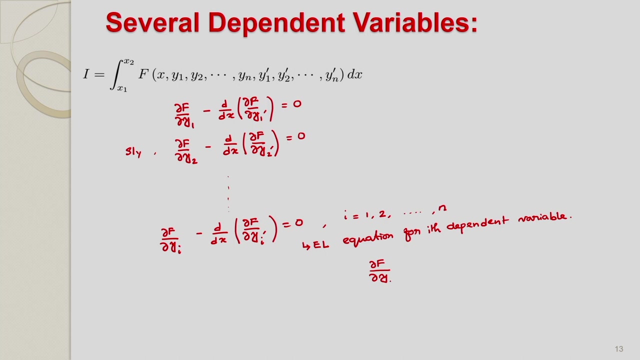 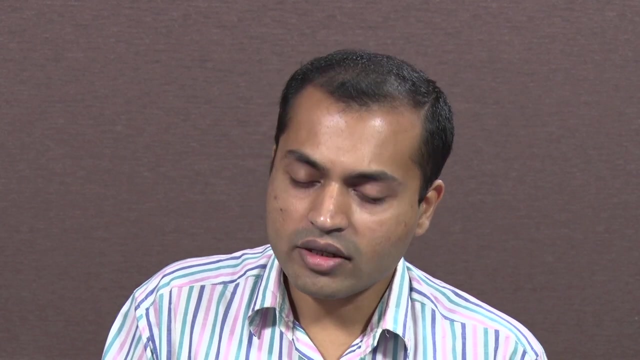 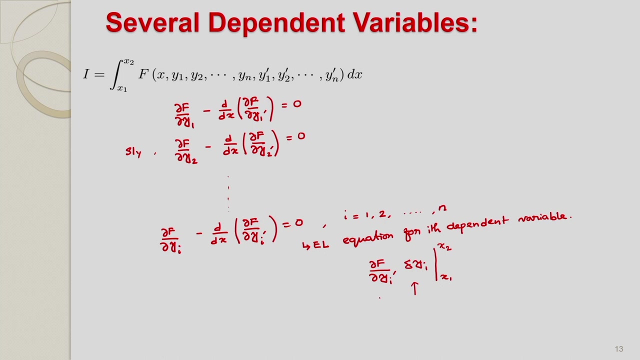 we have n differential equation. So in general we have for ith dependent variable, where i equal to 1 to n. So this is Euler Lagrange equation for ith dependent variable And we have in the similar way, I will have a gamma and gamma n. 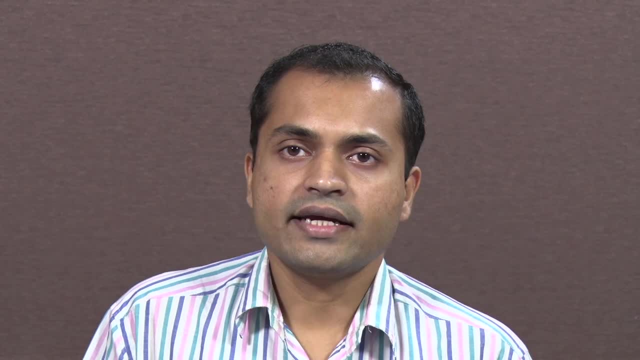 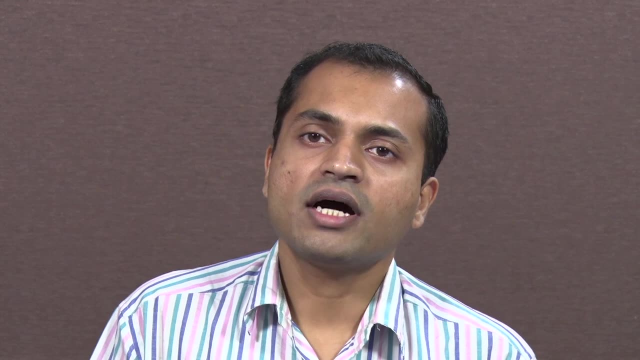 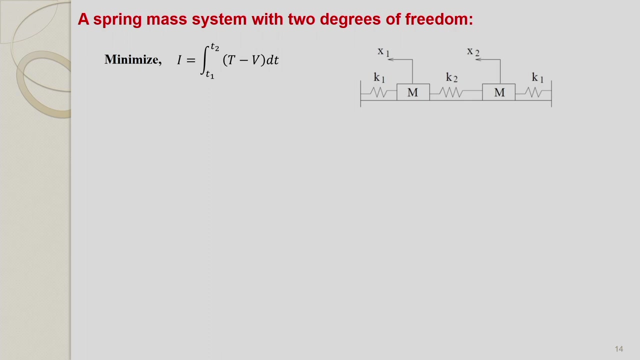 So this is n Euler Lagrange equation. We will understand this concept of several dependent variable using one example. There are two mass connected by 3 spring. Mass 1 has displacement x1, mass 2 has displacement x2.. 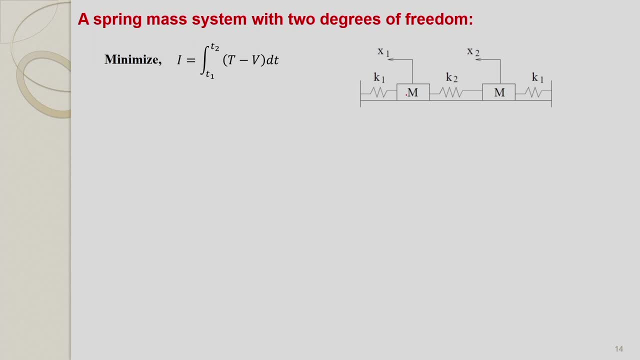 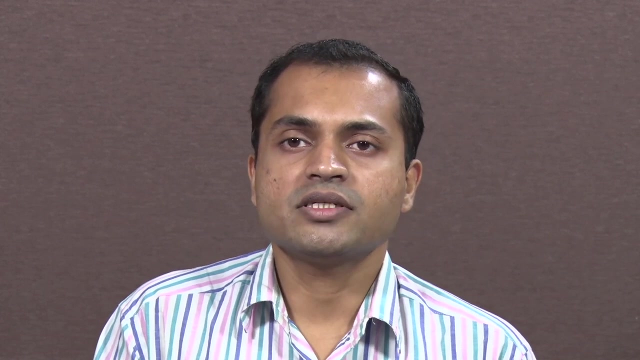 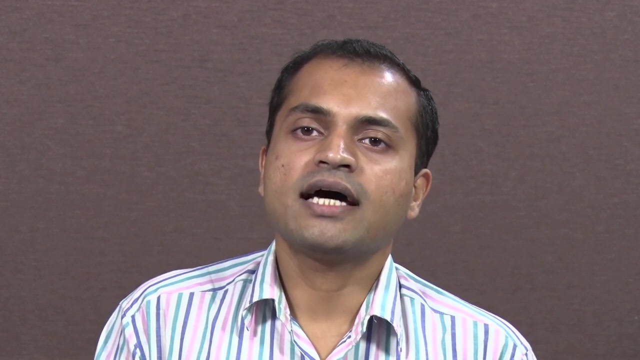 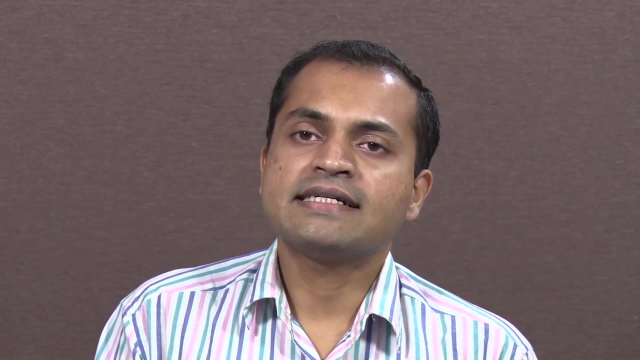 the governing differential equation for the motion of these two degree of freedom system. Here we will use Hamiltonian principle. When some particles are in motion under the action of conservative forces, then Hamiltonian principle tells us that the motion will happen such 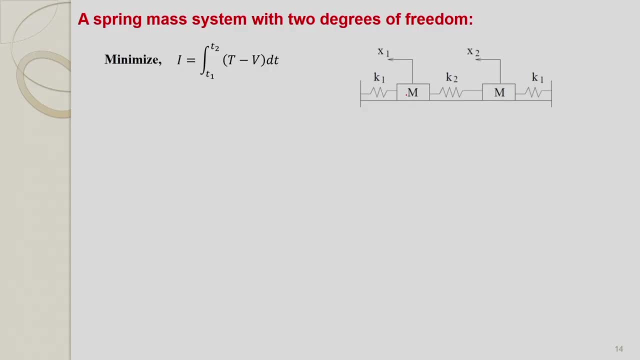 that it minimize Hamiltonian which is given by this functional. where T is total kinetic energy of the system of particles And V is total potential energy For this system, we can write the total kinetic energy as half m x1 dot square. Here our independent variable is time. It is time and there are two dependent variable. 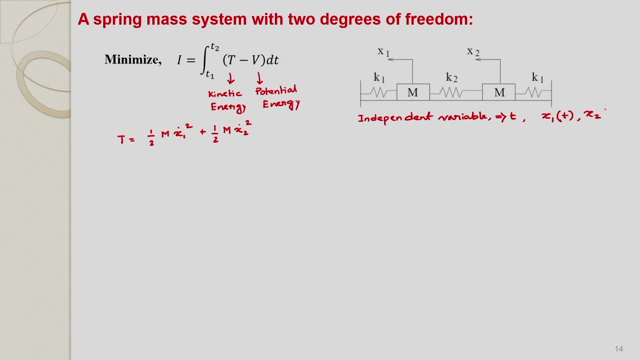 x1 and x2. And x2.. They both are function of independent variable time. We want to find governing differential equation of x1 and x2.. So this is our total kinetic energy, Now total potential energy for spring: 1.. 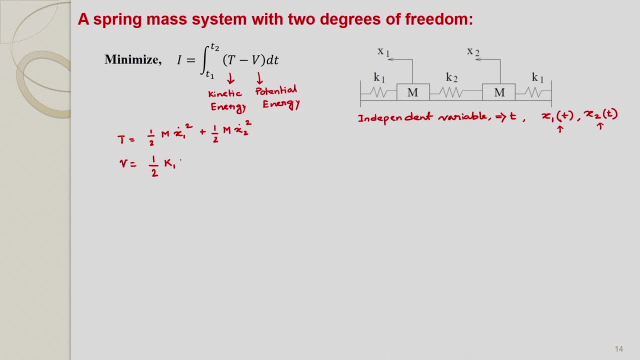 Now for spring 2, the total deformation is x1 minus x2.. And for spring 3, this is the stored energy. 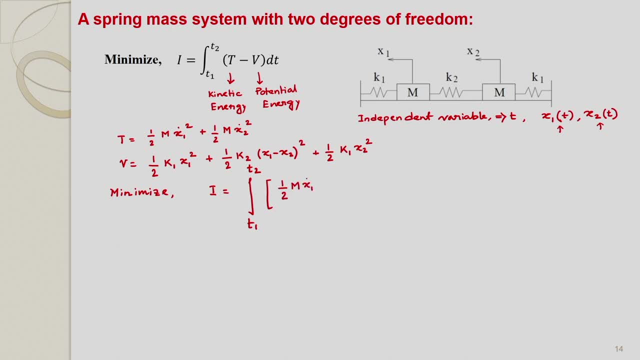 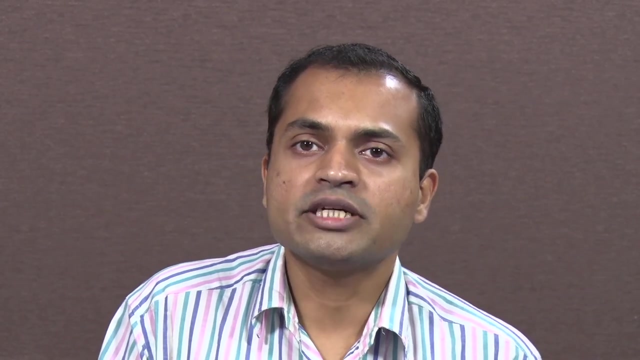 Total kinetic energy Minus total potential energy. So this is a functional which is function of. So this is a functional which is function of time. t, which is the independent variable function of x1 and x2. these are two dependent variable. So we have to minimize a functional which is function of two dependent variable. 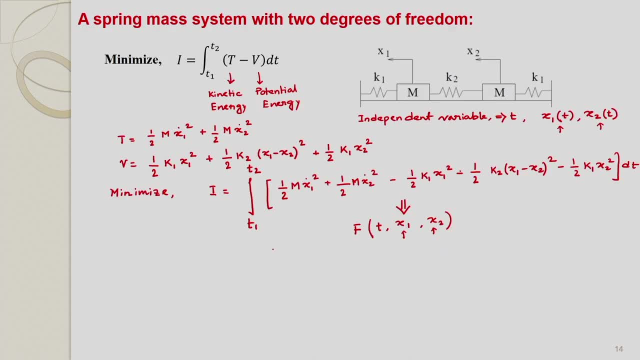 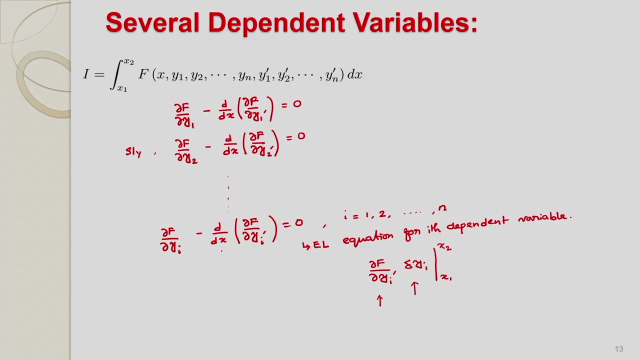 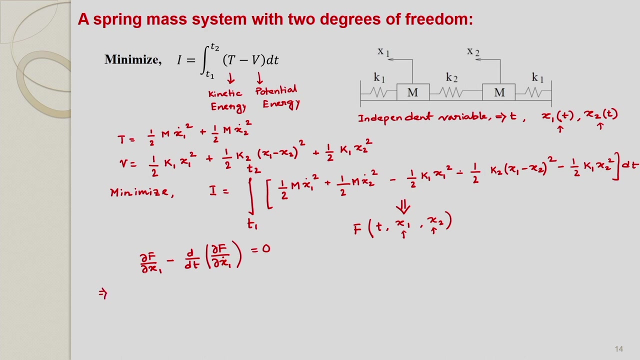 So this is our Euler Lagrange equation. So for this problem we can write Euler Lagrange equation for x1.. So here, if you see, independent variable is t and this is x1 dot. So for this functional, that del x1.. From this term: 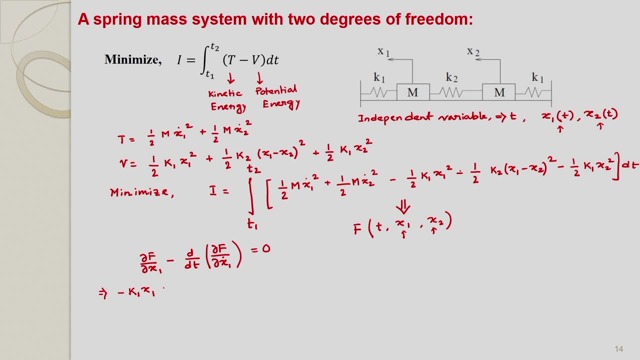 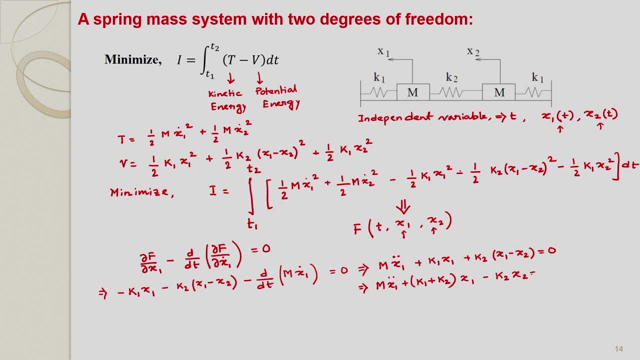 1. So this is our first governing differential equation. Now we have second Euler Lagrange equation for dependent variable x: 2. Therefore we can write: because of this minus, So this minus and this minus get canceled. 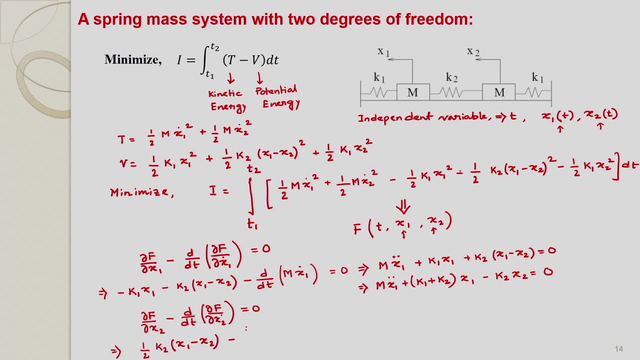 So So there will be 1, 2 will come. this will be k 1 x 2. again del f, del x 2 dot will give us m x 2 dot equal to 0.. So finally, m x 2 double dot plus. So for x 1, it will be: 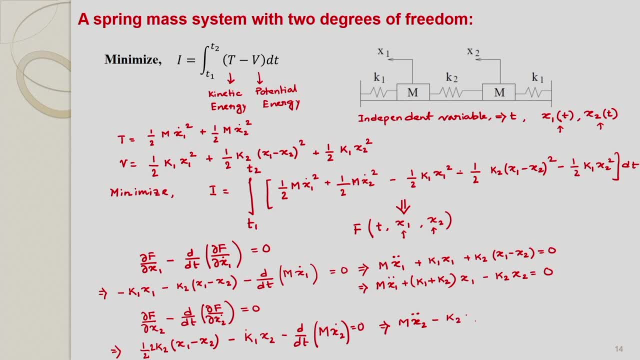 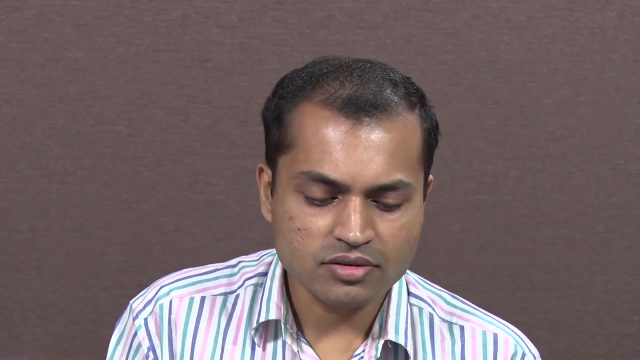 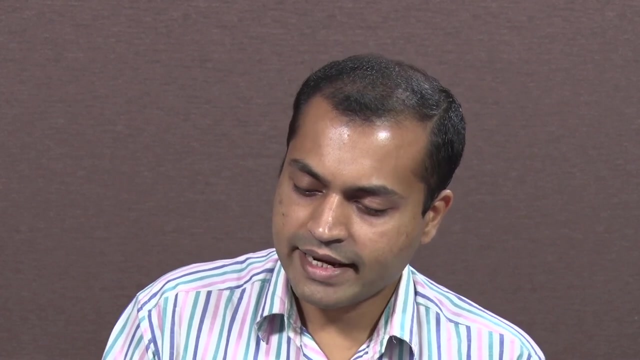 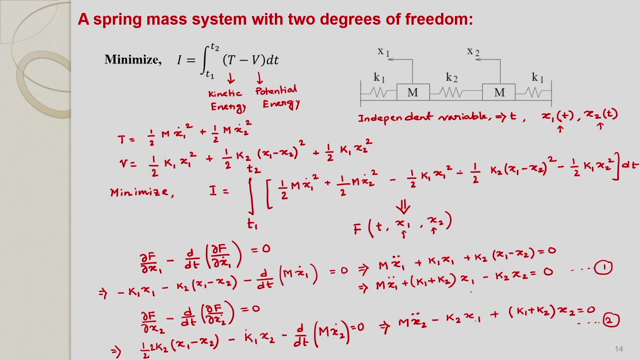 minus k 2 x 1.. Plus k 1 plus k 2 x 2, equal to 0.. So this is So you can see, after using Euler Lagrange equation for two dependent variables separately, we get two coupled differential equation of: